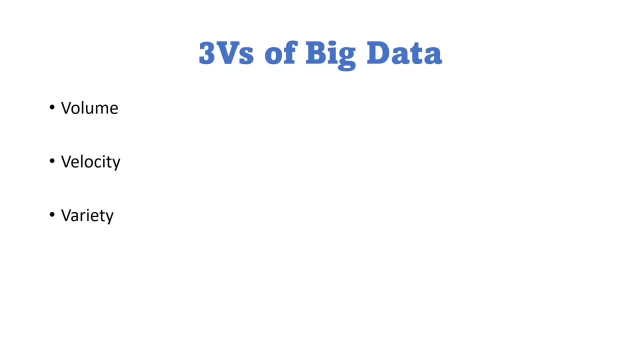 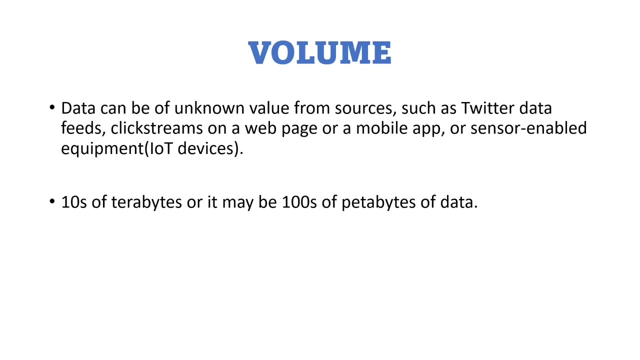 Let's now see about three Vs of Big Data. The three Vs of Big Data are Volume, Velocity and Variety. Now let's see about Volume. Data can be of unknown value from sources such as Twitter data Data feeds, clickstreams on a web page or a mobile app, or sensor-enabled equipment like IoT. 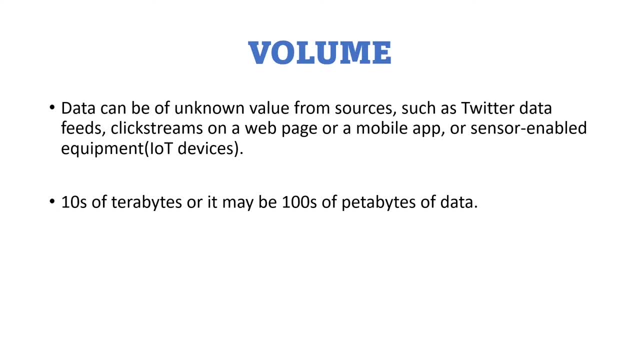 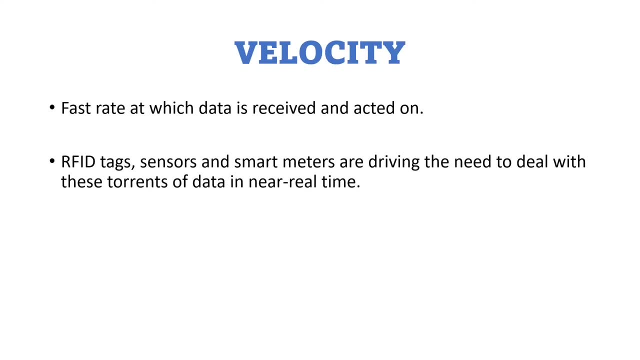 devices. For some organizations this might be tens of terabytes of data. For others it may be of hundreds of petabytes of data. Let's now see about Velocity. Velocity is the fast rate at which data is received and acted on. Data streams into businesses at an unprecedented speed and must be. 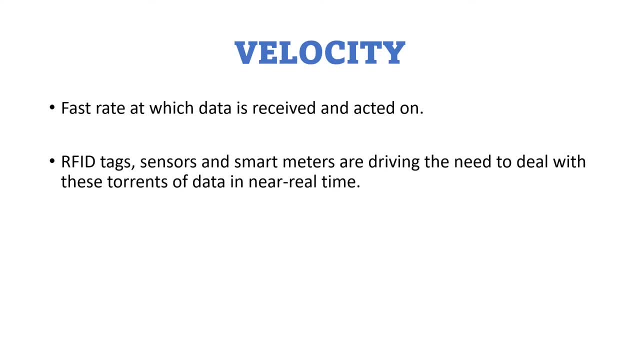 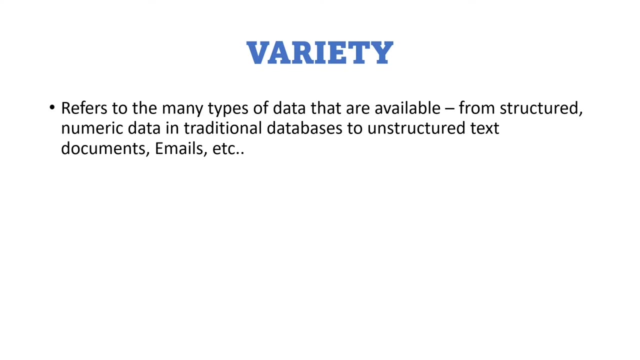 handled, In other words, data can be used in a timely manner. RFID tags, sensors and smart meters are driving the need to deal with these torrents of data in near real time. Talking about Variety, it refers to the many types of data that are available from structured 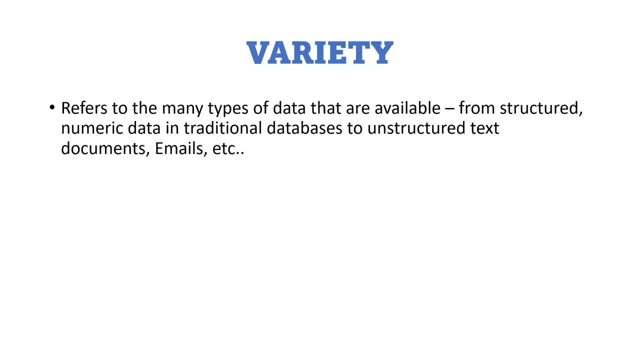 numeric data in traditional databases to unstructured text documents, emails, videos, audios, stock ticker data and financial transactions. We have two more Vs. It refers to value and veracity. Now let's see them one by one. We have a range of various products, and each comes with its own advantages and disadvantages. 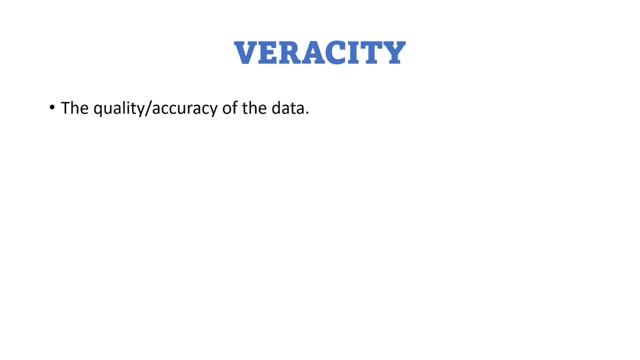 Variety is nothing but the quality or accuracy of the data. Since the data is collected from multiple sources, we need to check the data for accuracy before using it for business insights. This is the most important of all: the Vs, The bulk of data having no value is of no good to the company and less would be any market. 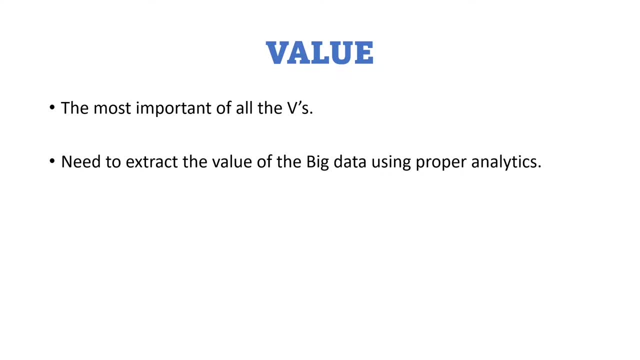 you turn it into something useful. we need to extract the value of the big data using proper analytics. now let's see about the benefits of big data: better decision making. many businesses, including travel, real estate, finance and insurance, are mainly using big data to improve their decision making capabilities, since big data reveals more information in an usable format. 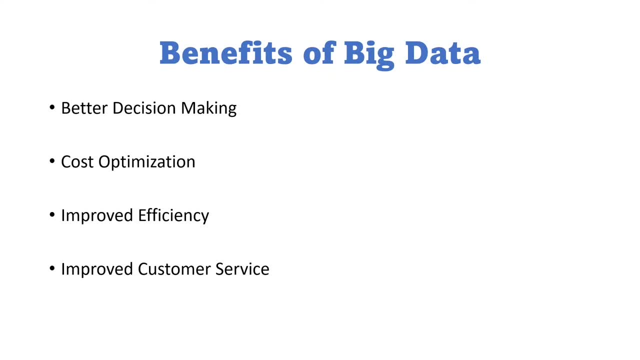 businesses can utilize that data to make accurate decisions on what customers want or not, on their behavioral tendencies. the next benefit is cost optimization. the logistics industry presents an excellent example to highlight the cost reduction benefit of big data. usually the cost of product returns is 1.5 times greater that of actual shipping costs. analyzing the big data allows 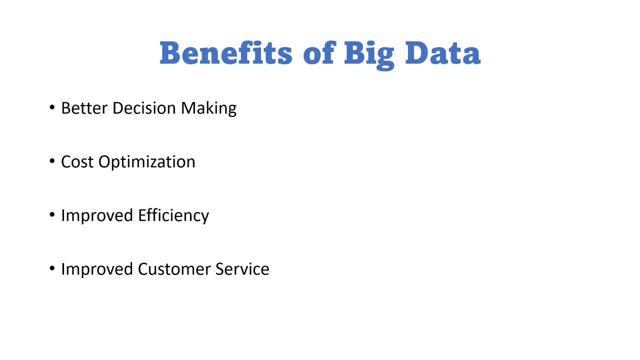 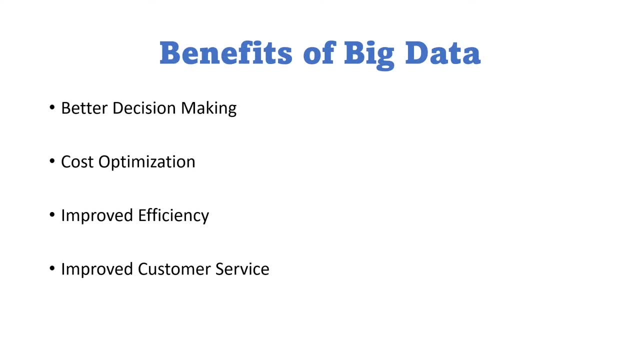 companies to take suitable measures to reduce losses on returns. next is improved efficiency by interacting with customers and gaining their valuable feedback. big data tools can gain large amounts of useful customer data. this data can then be analyzed and interpreted to extract meaningful patterns hidden within, which allows companies to create personalized products. the 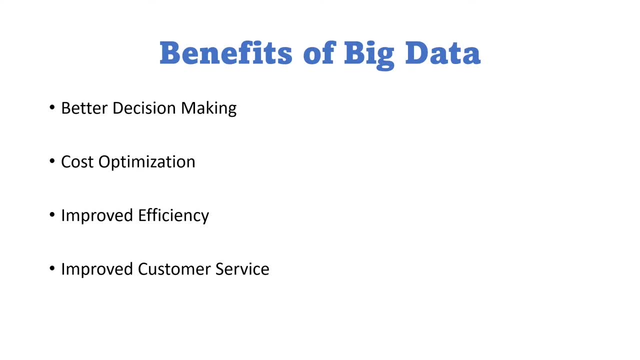 next is improved customer service. big data helps companies understand how their customers think and feel and thereby offer them more personalized products and services. offering a personalized experience can improve customer satisfaction, enhance relationships and, most of all, build loyalty. so far we have seen about the benefits of big data. let's move on to see what is big data analytics. 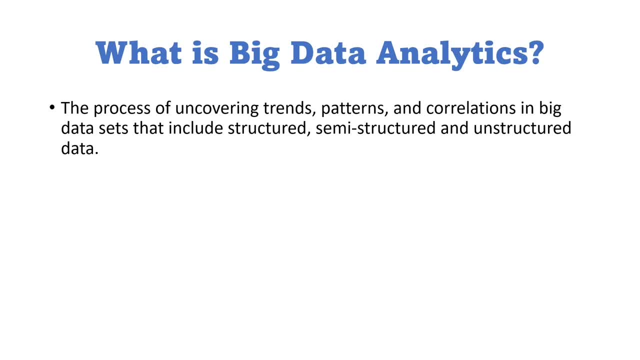 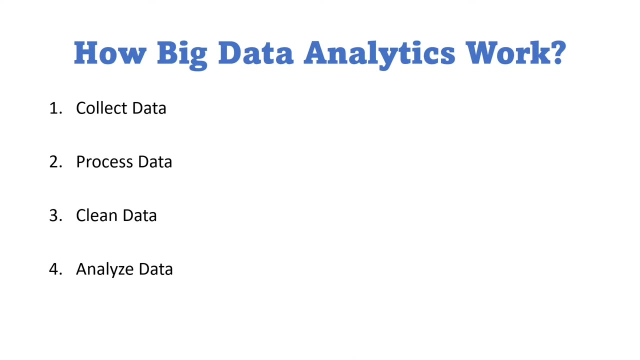 big data analytics describes the process of uncovering trends, patterns and correlations in big data sets that include structured, semi-structured and unstructured data. so now let's see how big data analytics work. the first process is to collect data, and the second is process data, and the third one is to clean the data. and fourth one: 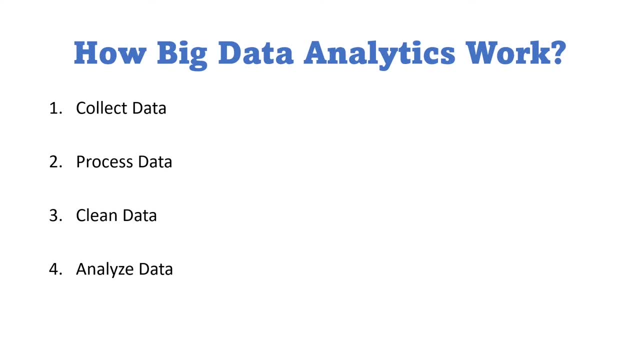 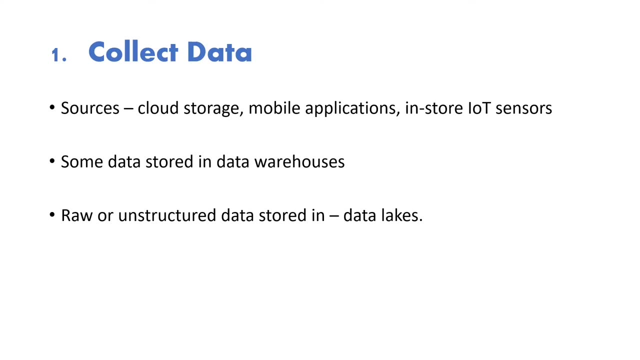 is to analyze data. let's see one by one. now let's see about collect data. with today's technology, organizations can gather structured and unstructured data from a variety of sources, like cloud storage, mobile applications, in-store iot sensors, etc. some data will be stored in data warehouses. store iot sensors, etc. some data will be stored in data warehouses, firework servers, ocd Center and so on. data storage softwares- site storage: sdf, sdf, sdf, sdf, inch Tenant sdf, sdf, sdfs, sdf, sdf, service sdf, sdf, sdf. current 중국 and other similar warehouse and platform related high performance products such as data storage software. 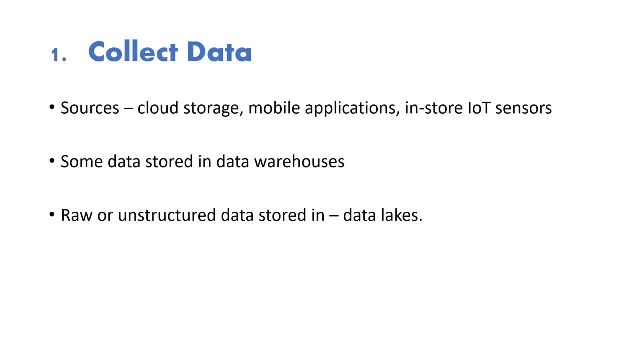 some data will be stored in data warehouses and those standard computers. data storage centers are stored in free devices such asömerexpress. Hash doesn't require a toast distribution of that data from the network stored in data warehouses- raw or unstructured data that is too diverse or complex for a 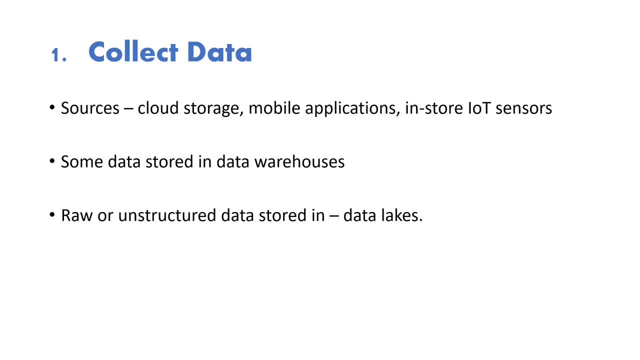 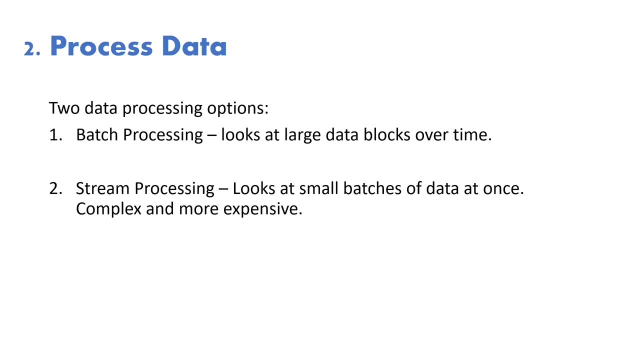 warehouse can be stored in a data lake. Next step is process data. Once data is collected and stored, it must be organized properly to get accurate results on analysis, especially when it's large and unstructured. Two data processing options are commonly used. 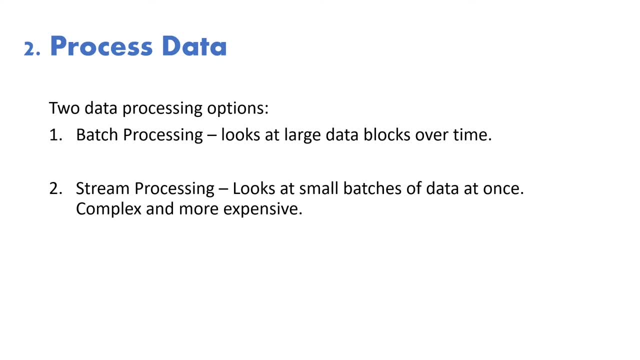 One is batch processing, which looks at large data blocks over time. Batch processing is useful when there is a longer turnaround time between collecting and analyzing data. Other one is stream processing, which looks at small batches of data at once, shortening the delay time between collection and analysis. 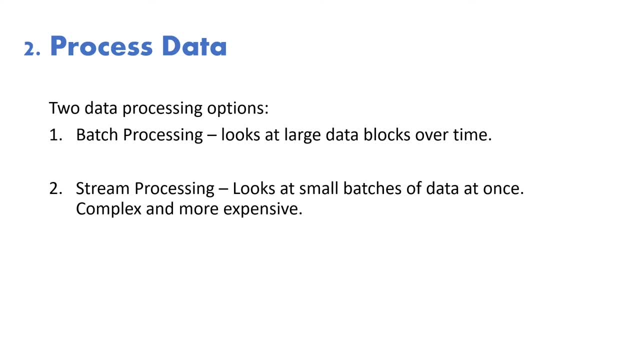 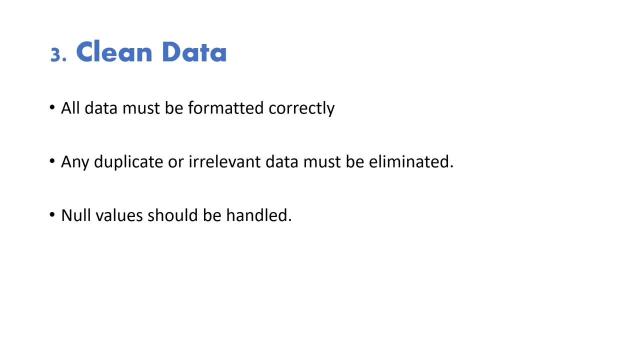 Stream processing is more complex and often more expensive. Next, let's see about clean data. Data, no matter big or small, requires cleaning. to improve data quality and get stronger results, All data must be formatted correctly. Any duplicate or irrelevant data must be eliminated. 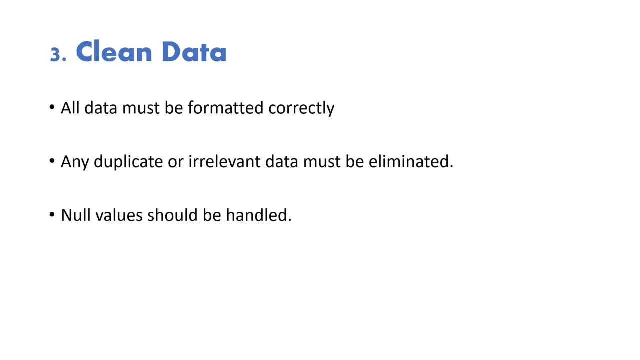 Null values should be handled. Last one is: analyze data. To get useful insights, we analyze the data. Some of those analytic methods include data mining, predictive analytics and deep learning. Data mining sorts through large datasets to identify patterns and relationships by identifying. 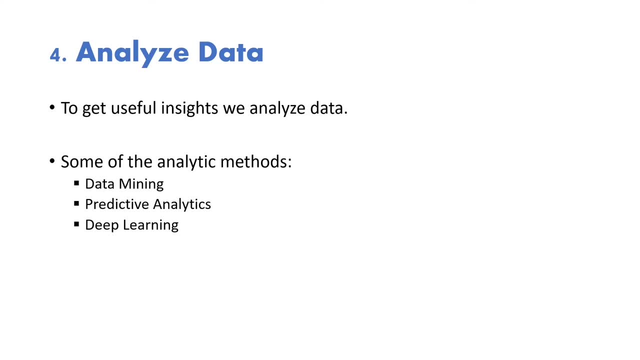 anomalies and creating data clusters. Predictive analytics uses an organization's historical data to make predictions about the future, identifying upcoming risks and opportunities. Deep learning imitates human learning patterns by using artificial intelligence and machine learning to layer algorithms and find patterns in the most complex way. 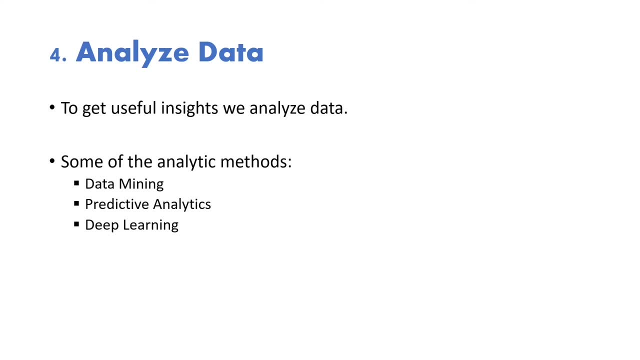 Big data analytics cannot be narrowed down to a single tool or technology. Instead, several types of tools work together to help you collect, process, cleanse and analyze big data. We'll learn about them in the upcoming videos. Now let's see why big data analytics